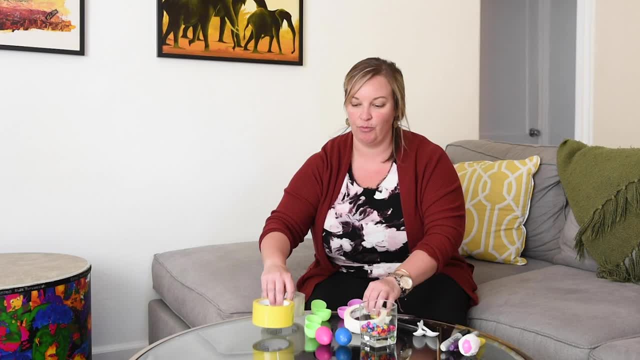 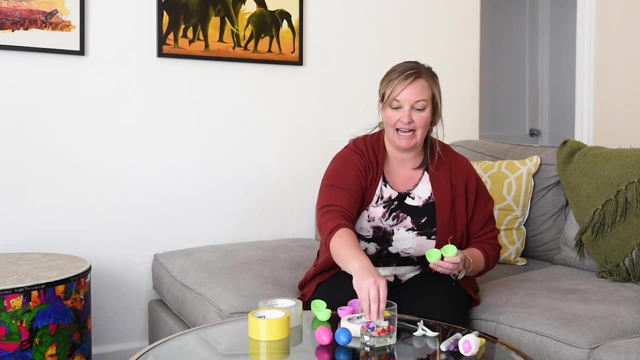 you can sort of think about the age of your kiddo and what your kiddo would work best with. So the first thing we're going to do is we're going to take our eggshell and we're going to put some beads inside. A great opportunity for counting, a great opportunity to take. 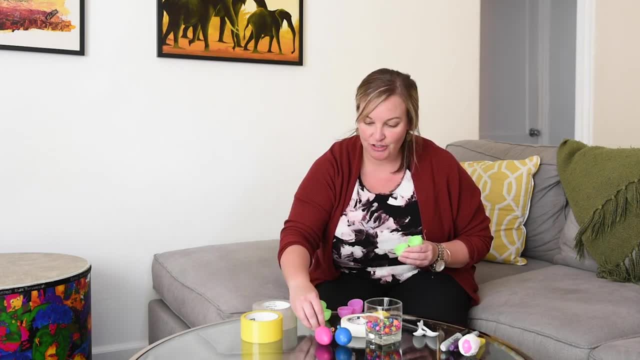 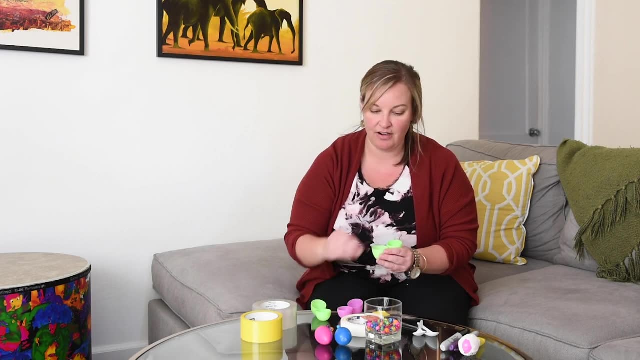 some beads and decide what colors we want. I'm going to do some orange and green together and in this one I'm going to put five ones: One, two, three, four, five. I'm going to close that up, get a nice seal on it and listen. 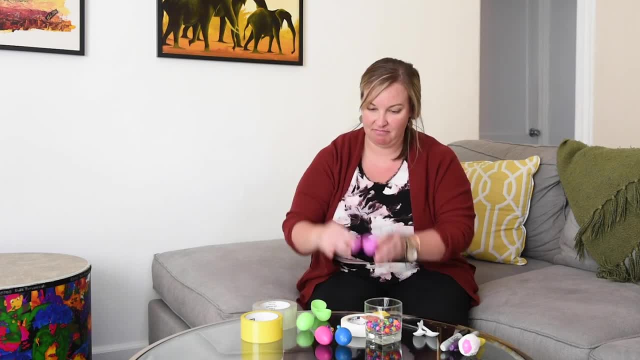 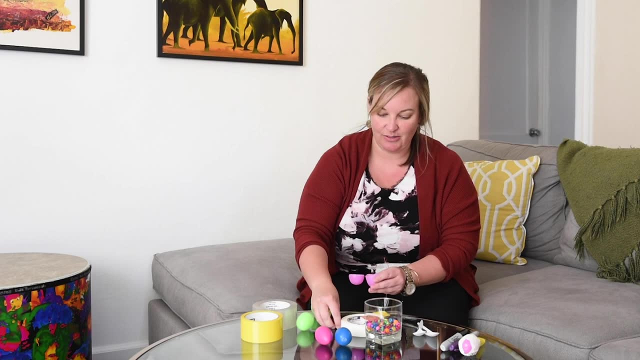 to it Not bad. In another one I'm going to increase the number by a lot. So I'm going to say I'm going to put 15 in and we're going to do this with any colors that we want, Your. 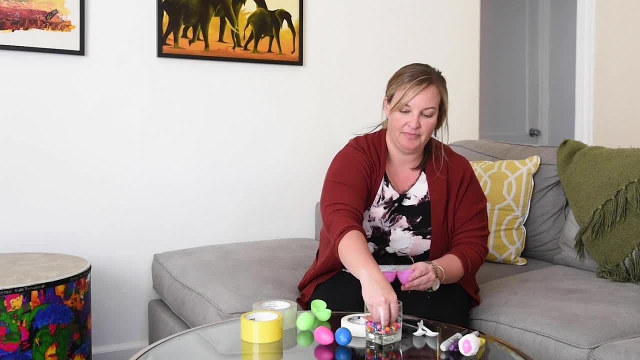 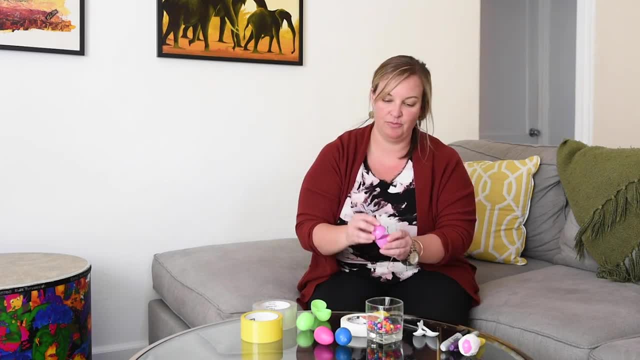 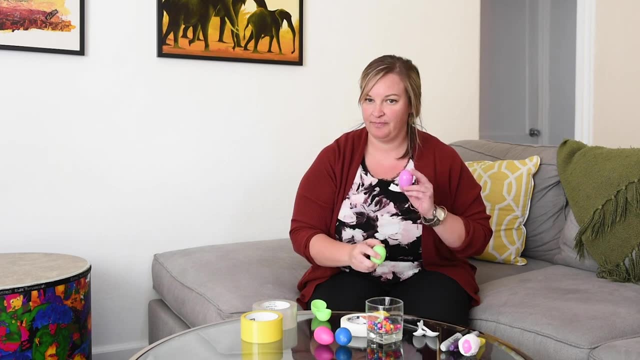 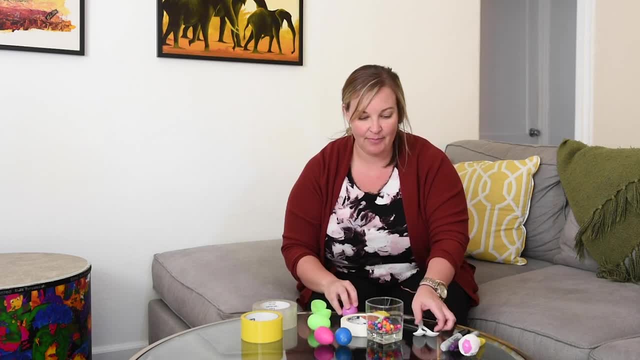 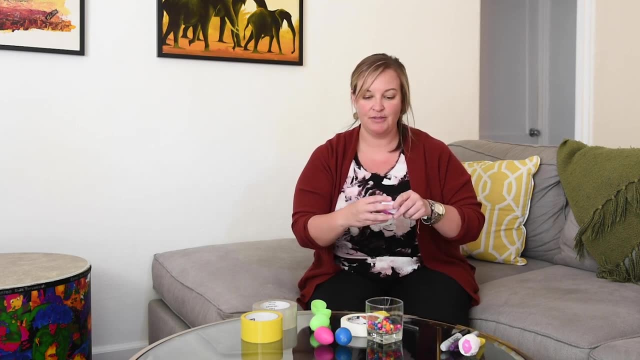 have a different sound about them. The next step is we're going to take our two spoons. We're going to put our egg shaker right in the middle of those two spoons. Now, depending on the age of your child, this is where you may need to help them, and that would be a great opportunity for you to use your hands, your hands, your hands- Oh, I love handaways. On Nook & Nook, we're using our handaewoods. brought assistance here where our hands are Tropical Awesome. On Pr spotted microwave oven: I love nooks and nooks and powder. 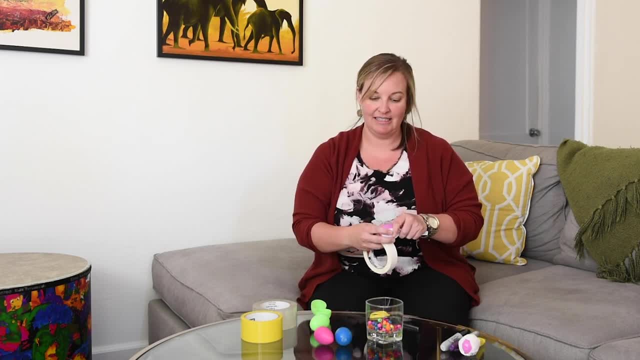 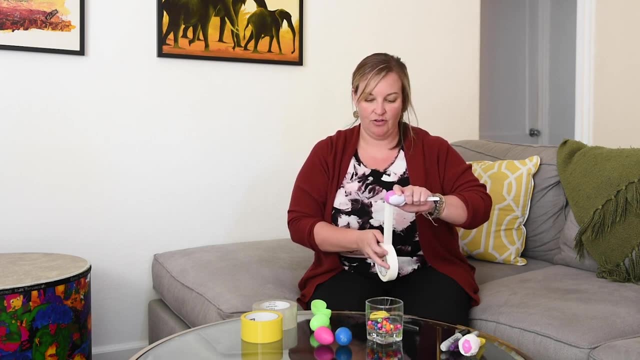 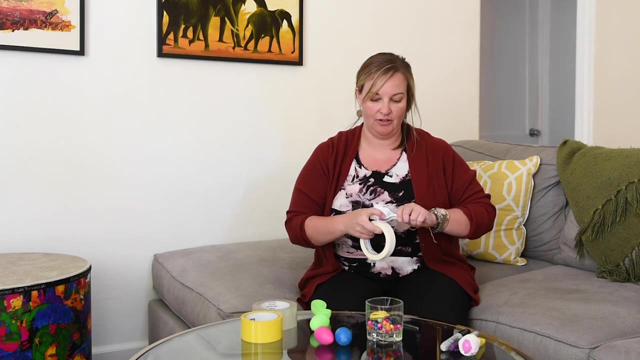 hands while they take their hands, and either using masking tape, which i think is great for our youngest kiddos because we don't have to worry about tearing it. if you give them a little piece, they can either wrap it around or they can just tape it. but we want to start with the top here. 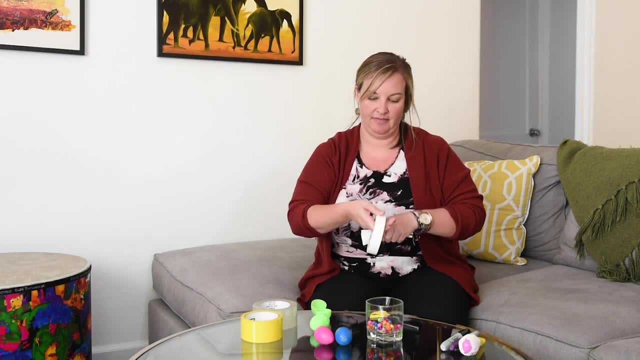 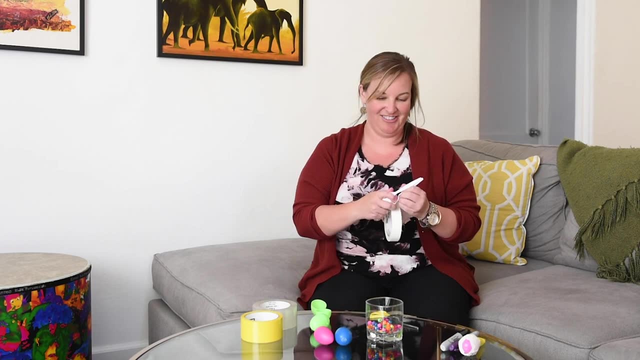 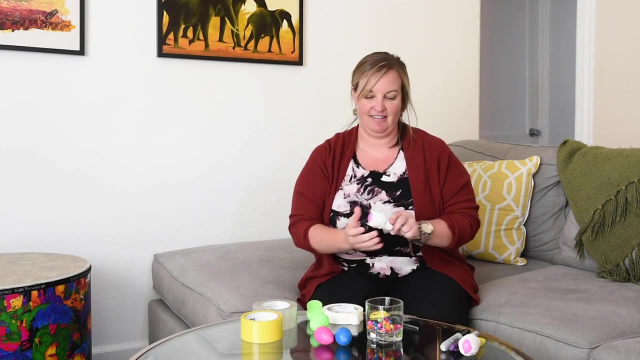 so that we get it nice and secure now. if you've taken classes with me at mim, you know that my preference would be for more tape. so once you get going with just a little bit of tape, you can just take it around. it doesn't matter how pretty it looks, because we can decorate it.